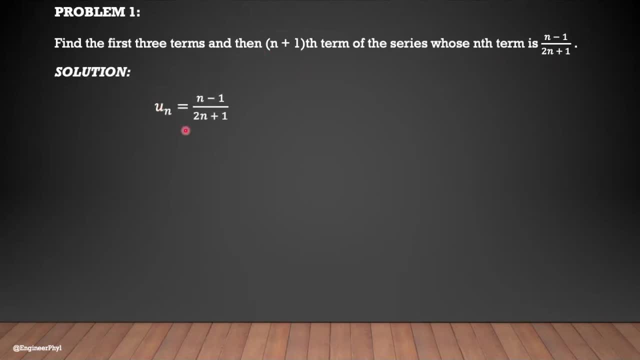 For our solution, let us write our nth term: u sub n is equal to n minus 1 over 2n plus 1.. Now here, since we are asked to solve for the first three terms and the n plus 1 term, we are going to replace n by for our first term. 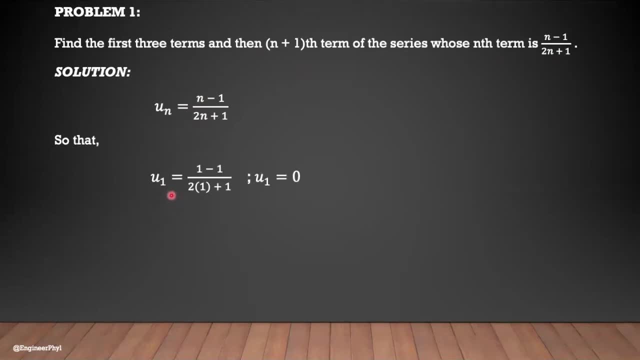 n equal to 1.. 1, our u sub 1,, or the first term is equal to 1 minus 1 over 2 times 1 plus 1.. Our first term is equal to 0.. Now for our second term, where n is equal to 2,, we have 2 minus 1 over 2 times 2. 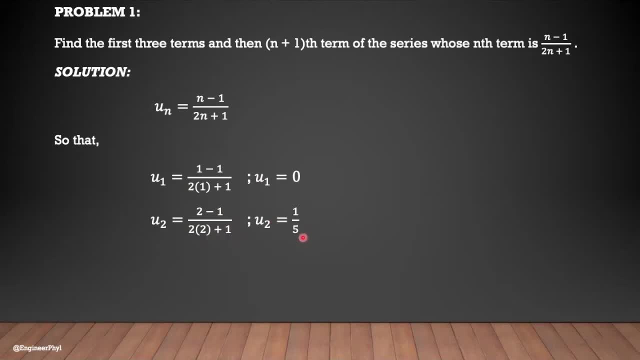 plus 1.. Our second term is 1 over 5.. And for the third term where n is equal to 3, this is 3 minus 1 over 2 times 3 plus 1.. So our third term is 2 over 7.. Now for the n plus 1 term. 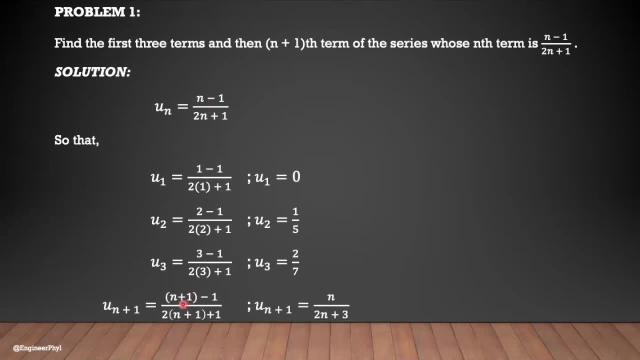 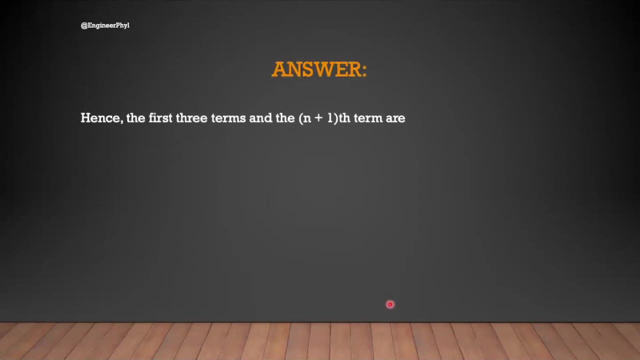 replacing n by n plus 1, we have the n plus 1 minus 1 over 2 times. the quantity n plus 1 plus 1 is n over 2n plus 3.. Now the first three terms and the n plus 1 term are 0, 1 over 5,. 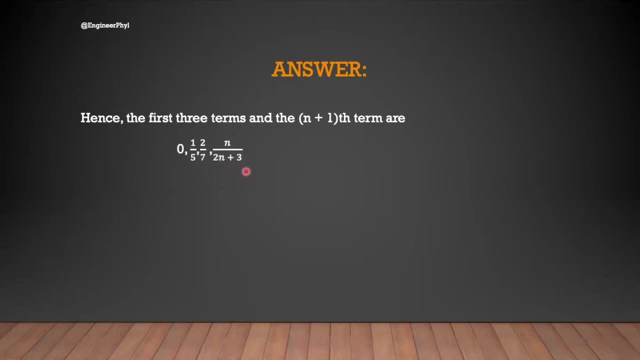 2 over 7, and n over 2n plus 3 as our n plus 1 term. Now, if you are asked to express your answers in terms of the infinite series, so taking note that the infinite series u sub 1 plus u sub 2, 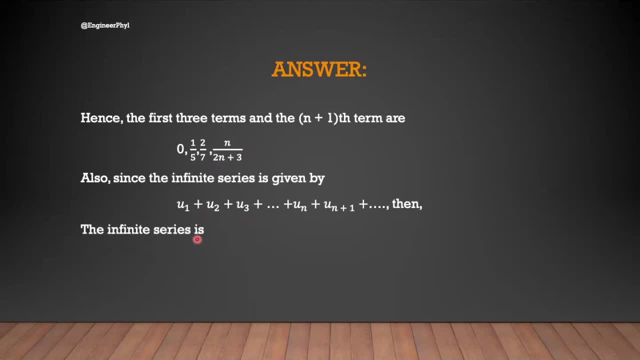 plus u sub 3, and so on. Then the infinite series will be 0 plus 1 over 5, plus 2 over 7, plus you have the ellipses. our nth term is n minus 1 over 2n plus 1, plus the n plus 1 term, which is n over 2n plus 3.. 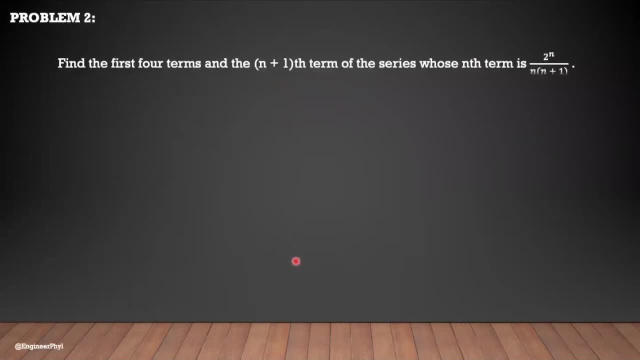 Let's go to example number two. We find the first four terms and the n plus 1 term of the series whose nth term is 2n or 2 raised to n over n times n plus 1.. First we write u sub n equal to 2 raised to n over n times n plus 1.. It follows that at n equal 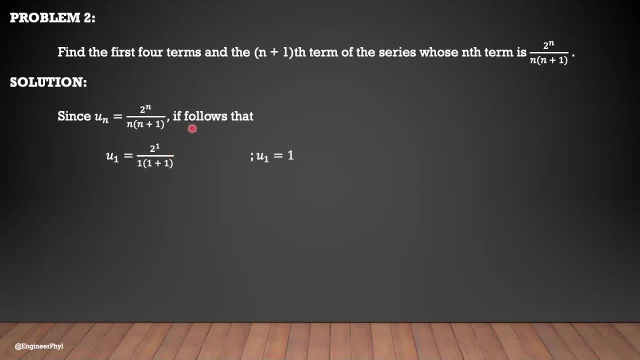 to 1,. our first term is 2 raised to 1, over 1 times the quantity 1 plus 1.. We have 1 as our first term For n equal to 2,. our second term is 2 raised to 2, that is 4, over 2 times 2 plus 1,. 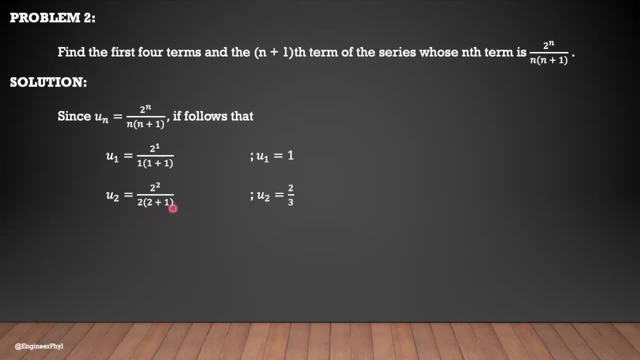 so this will be 6.. So 4 over 6 will be, if we simplify, the answer is 2 over 3.. Now for our third term, where n is equal to 3, it will be 2 raised to 3 over 3 times 3 plus 1.. 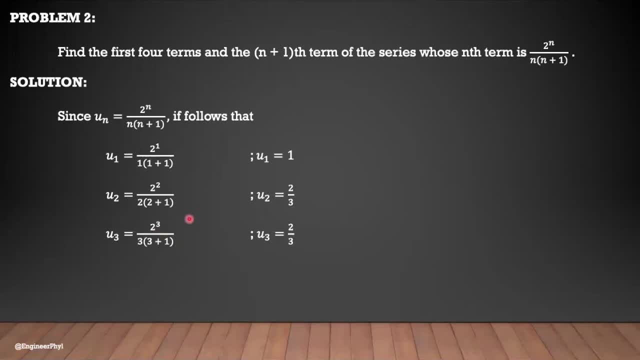 Now, 2 raised to 3 is 2 raised to n over n times n plus 1.. So 2 raised to n over n times n plus 1.. 2 raised to 3 is equal to 8, 8 divided by so here 4 times 3, is 12.. So 8 over 12 is equal to 2 over 3.. 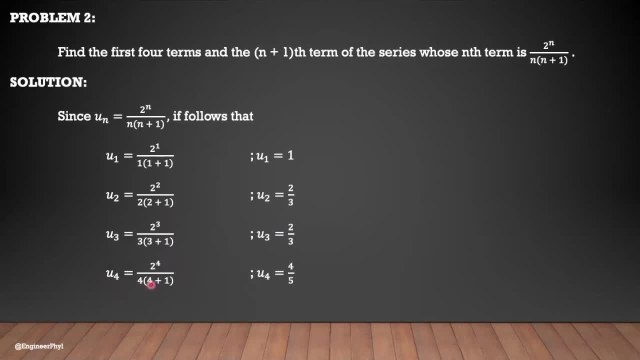 Now for our fourth term, where n is equal to 4, 2 raised to 4 over 4 times 4 plus 1.. If we simplify this, the answer is 4 over 3.. Now for the n plus 1 term, or our use of n plus 1.. Replacing n by n plus 1, we have 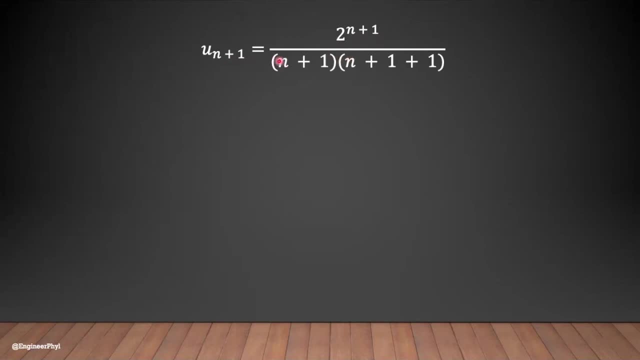 this expression, 2 raised to n plus 1, over the quantity n plus 1, times n plus 1 plus 1, or basically multiplying n plus 1 by n plus 2.. So we have n squared plus 3, n plus 2.. 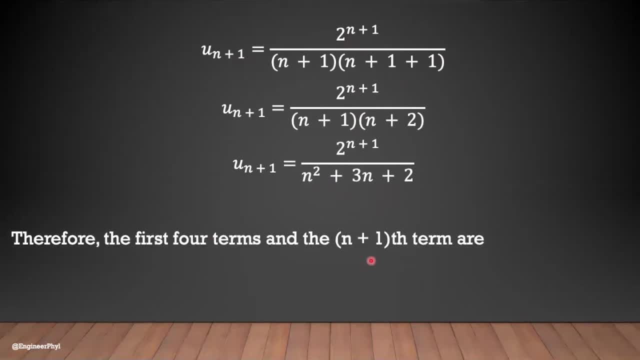 Therefore, the first four terms and the n plus 1, are n plus 1 times n plus 1 times 3 n plus 2.. So we have n squared plus 3, n plus 2.. term are 1, 2 thirds, 2 thirds, 4 over 5, 2 raised to n plus 1 over n squared plus 3n plus 2.. 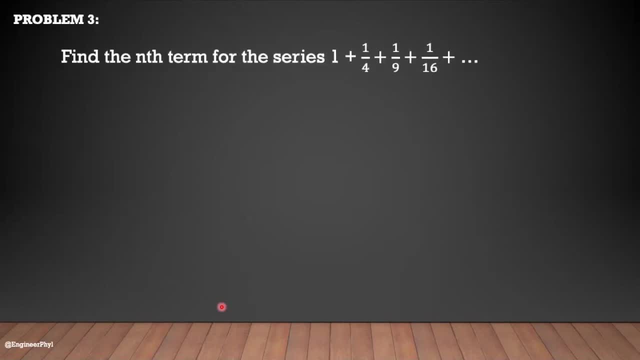 Example number 3. Find the nth term for the series: 1 plus 1 over 4, plus 1 over 9, plus 1 over 16, and so on. Now observing through the first four terms to establish the nth term, So since u sub 1 is equal to 1, so we can say that 1 over the square. 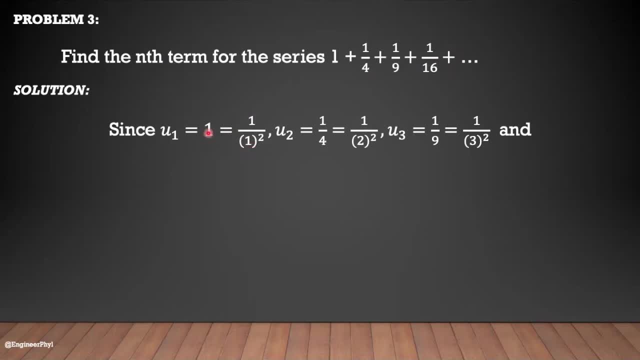 of n is equal to 1.. Now for our second term, which is 1 fourth, or 1 over 4, it is equal to applying the same idea for our first term. So 1 over the square of our n, equal to 2,. 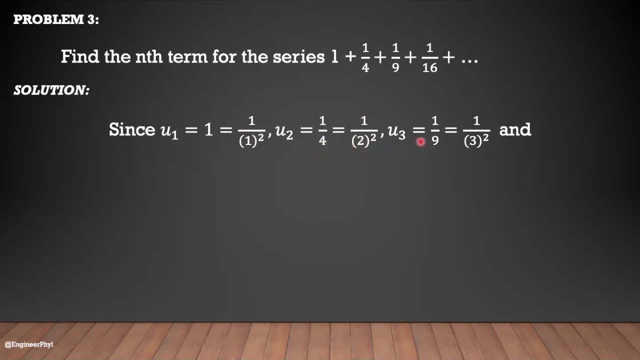 2 is 4.. For our third term, where n is equal to 3, so 1 over 3 squared is equal to 1 over 9.. And for our fourth term, where n is equal to 4, so 1 over 4 squared is 1 over 16,. 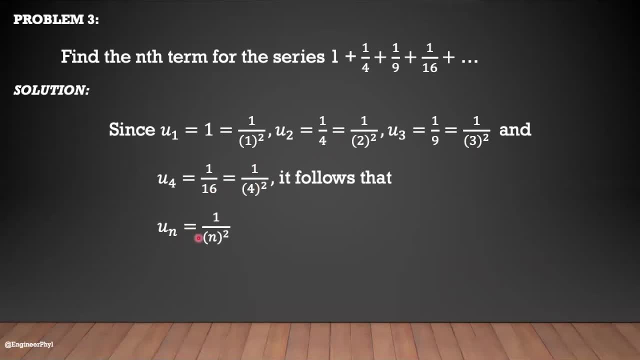 it follows that our nth term is equal to 1 over n squared. Therefore, our nth term, or our u sub n, is equal to 1 over n squared. Example number 4.. Find the nth term of the series 1 plus x over 2 factorial plus x squared. 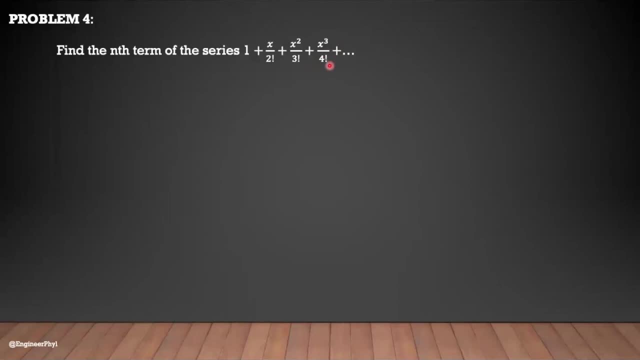 over 3 factorial, plus x cubed over 4 factorial and so on. So establish the nth term. Since u sub 1 is equal to 1, so we can say that x raised to 1 minus 1, so in this case x raised to 0 is 1,. 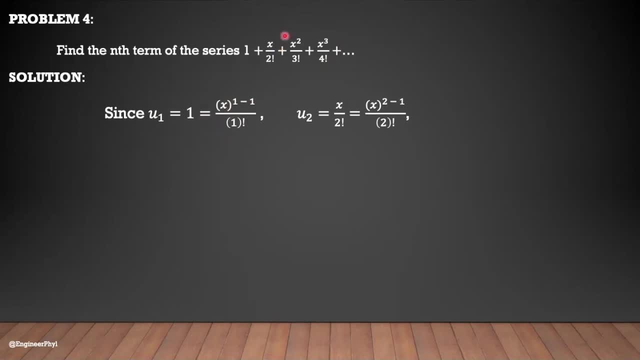 over 1 factorial is still equal to 1.. Observing through the second term, u sub 2, the same idea here. so x raised to our n is 2, so 2 minus 1 is 1, we have x. 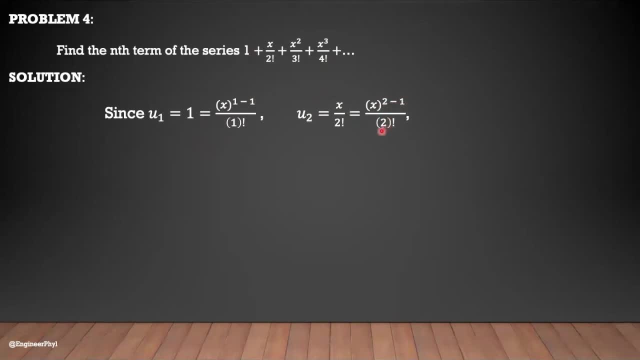 and n is equal to 2, so 2 factorial is equal to this term. Now for our third term serving the same idea. so x raised to 3 minus 1 is equal to x squared over 3 factorial. Now for our fourth term, at n equal to 4,. 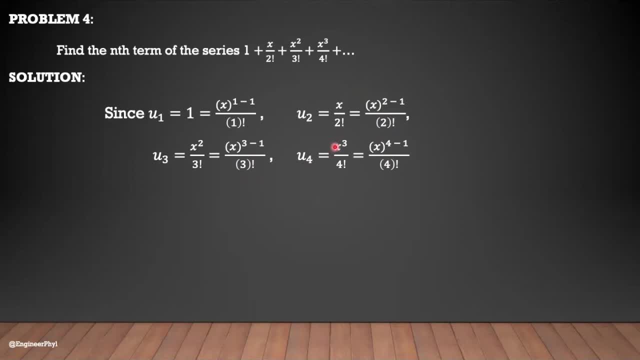 x raised to 4 minus 1 is equal to x cubed and we have n is equal to 4 for our denominator, so 4 factorial. It follows that our u sub n is equal to, or the nth term is equal to x raised to n minus 1 over n factorial. 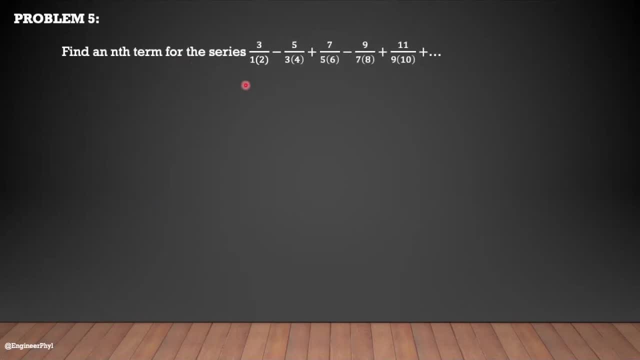 Problem number 5.. Find an nth term for this series: 3 over 1 times 2 plus 5 over 3 times 4, plus 7 over 5 times 6 minus 9 over 7 times 8, plus 11 over 9 times 10, and so on. 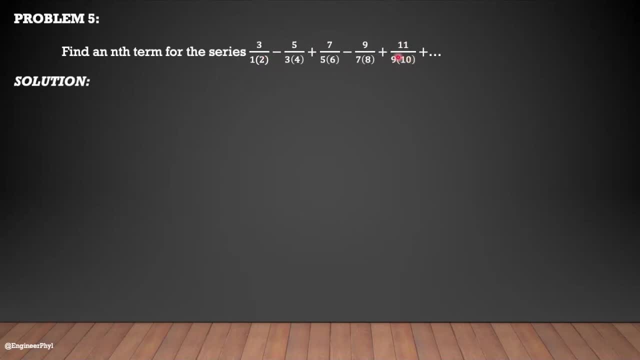 So observe that the series contains an alternating sign. Now this should be taken into consideration for writing or for determining our nth term, Since u sub 1 is equal to 3 over 1 times 2, and considering that n is equal to 1 here and having a positive sign, we have negative 1. 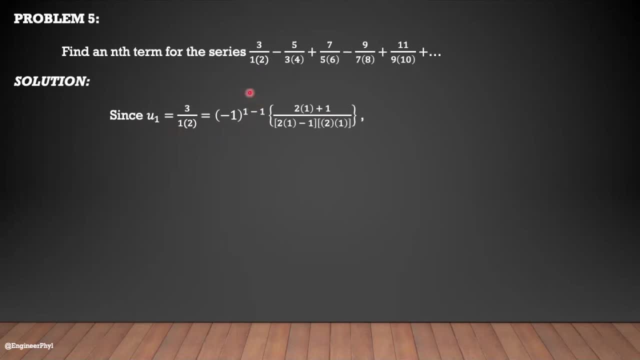 raised to 1 minus 1 to make this a positive sign. And for the numerator, which is 3, we can say that 2 times 1 plus 1 is equal to this value over. we have the factors 1 times 2.. 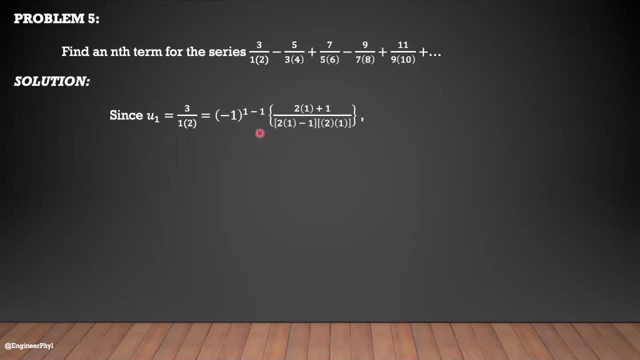 So for the first factor we can say: 2 times 1 minus 1 is equal to 1, and 2 times 1 is equal to 1.. So for the second factor we can say: 2 times 1 minus 1 is equal to 1,. and 2 times 1 is equal to 1.. So for the third factor we can say: 2 times 1 minus 1 is equal to 1, and 2 times 1 is equal to 1.. So for the fourth factor we can say: 2 times 1 minus 1 is equal to 1,. 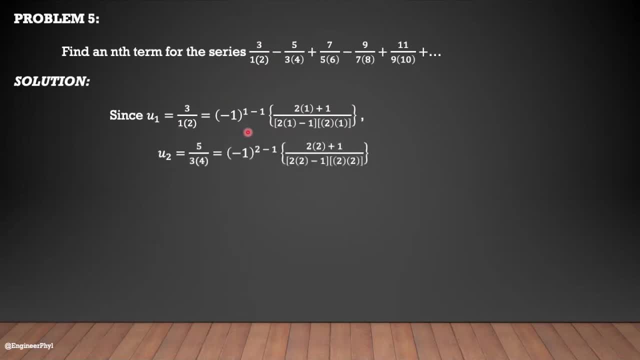 and 2 times 1 is equal to 1.. So for the fifth factor we can say: 2 times 1 minus 1 is equal to 1, and 2 times 1 is equal to 2.. Now let's observe the second term, which is 5 over 3 times 4.. 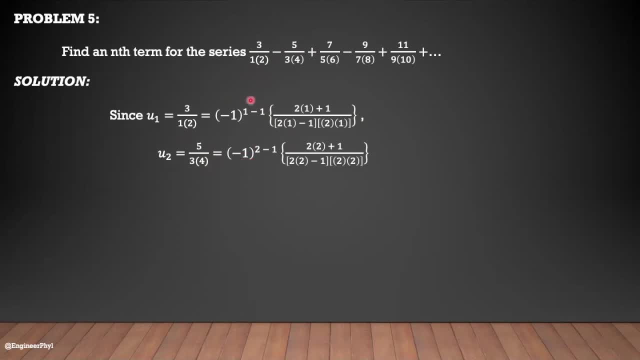 Now for the sign negative, we can say that negative 1, the same idea for our first term: negative 1 raised to 2 minus 1 will give us a negative sign. And for the numerator, which is 5, 2 times 2 plus 1 is equal to 5.. And for the first factor, the denominator, we have 2 times 2 minus 1. 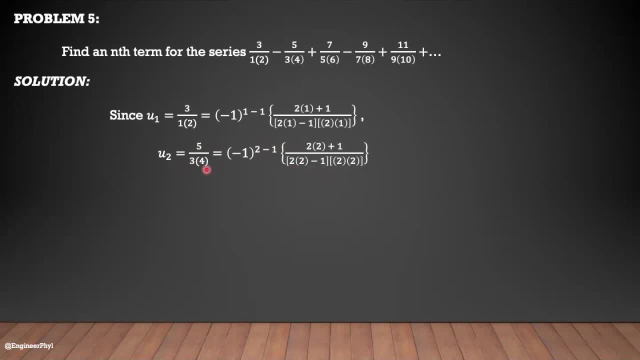 is 3, 2 times 2 is 4.. Observing this same idea for our third term: 7 over 5 times 6.. So this sign should be positive. So we can say negative: 1 raised to 3 minus 1.. 3 minus 1 is 2.. Negative: 1 raised to 2 is positive. 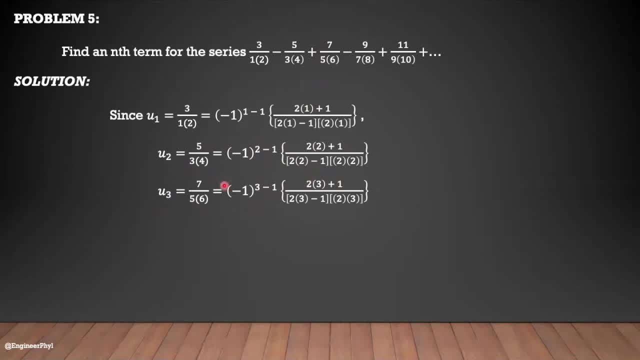 So the sign here is correct. For the numerator 7, we have 2 times 3 and is 3.. So 2 times 3, 6 plus 1 is 7.. And for the denominator, which is 5 times 6, for the first factor, 5,. 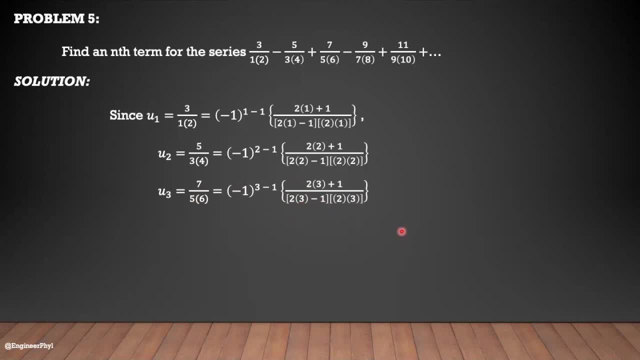 2 times 3, 6.. minus 1 is 5, correct and 2 times n equal to 3,, so 6, correct. Now for the fourth term, which is 9 over 7 over 8, and for the sine negative, we have negative 1 raised to 4 minus. 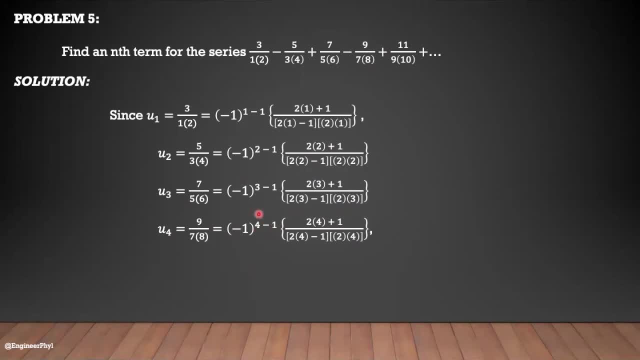 1,. 4 minus 1 is 3, negative. 1 raised to an odd number is negative, so the sine is correct. 2 times n equal to 4, so that's 8 plus 1 is 9, and for the denominator it should be 7. for the: 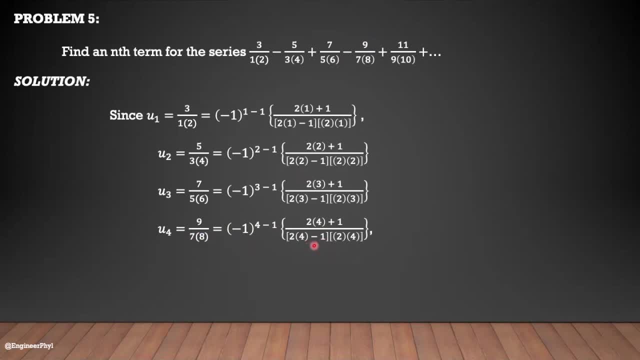 first factor. so 2 times 4 is 8, minus 1 is 7,, 2 times 4 is 8, and for the fifth term, positive sine. so negative. 1 raised to 5 minus 1 is positive For the numerator. 2 times 5 is 10. 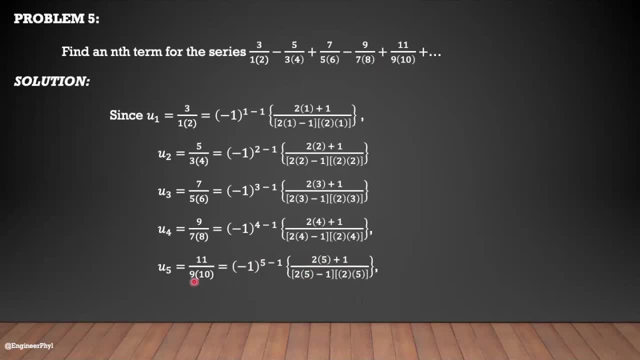 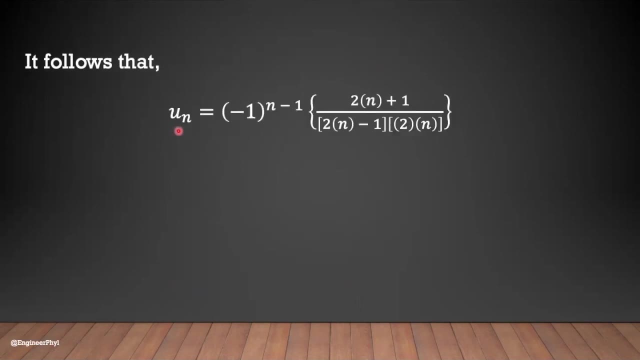 plus 1 is 11,. denominator should be 9 and 10,. so 2 times 5, n is equal to 5,. so 10 minus 1 is 9, and 2 times 5 is 10.. So we can say that our nth term, or u sub n, is equal to negative 1 raised to n minus 1. 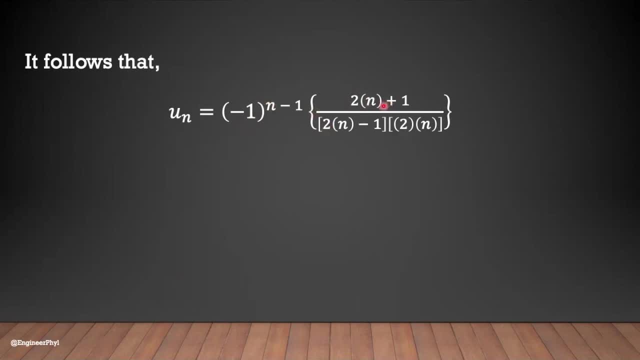 times the quantity for the numerator, 2 times n plus 1, over the quantity, 2 times n minus 1 for the first factor and 2 times n for the second factor. Therefore, this is our nth term: Negative 1 raised to n minus 1 is negative 1, and 2 times n for the second factor. 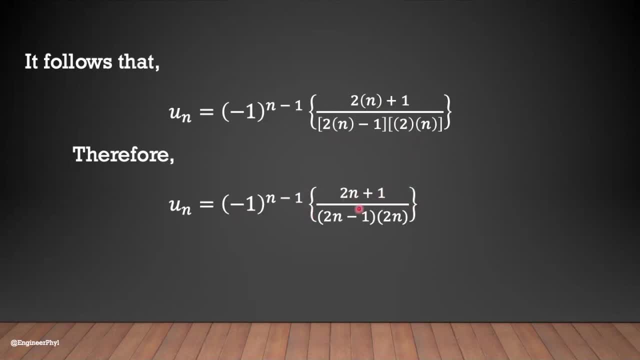 so negative: 1 raised to n minus 1 times 2n plus 1, over the product of 2n minus 1, and 2 times n. Inverses and groups. Let M star be a monoid with identity E. An element A in M is called invertible if there is an element B in M such that A star B equals B star A is equal to E. 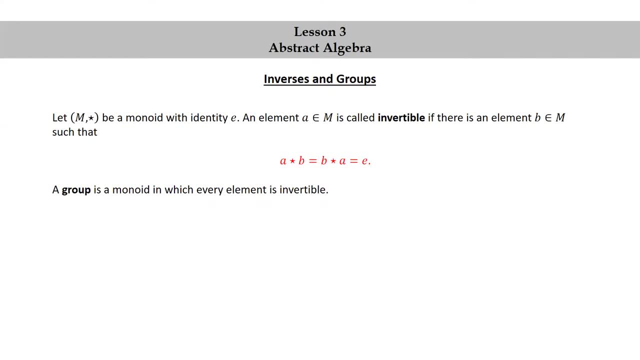 A group is a monoid in which every element is invertible. Groups appear so often in mathematics that it's worth taking the time to explicitly spell out the full definition of a group. So in other words I'm just going to repeat the definition of a group but I'm going to spell out all the details without using the word monoid. 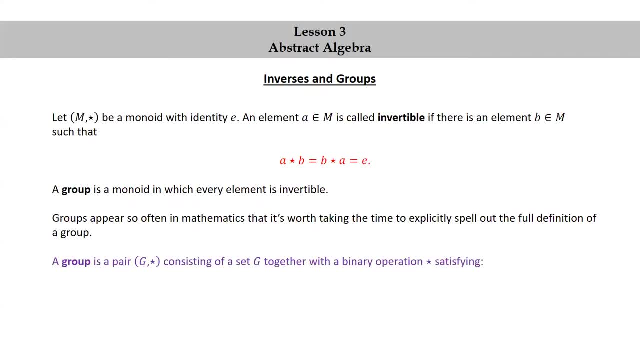 A group is a pair G star consisting of a set G together with a binary operation star satisfying one associativity for all the elements of the group. So a group is a pair G star consisting of a set G together with a binary operation star satisfying one associativity for all the elements of the group. So a group is a pair G star consisting of a set G together with a binary operation star satisfying X star Y star Z is equal to X star Y star Z. 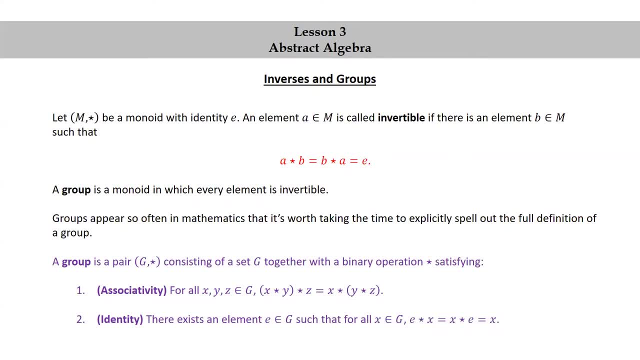 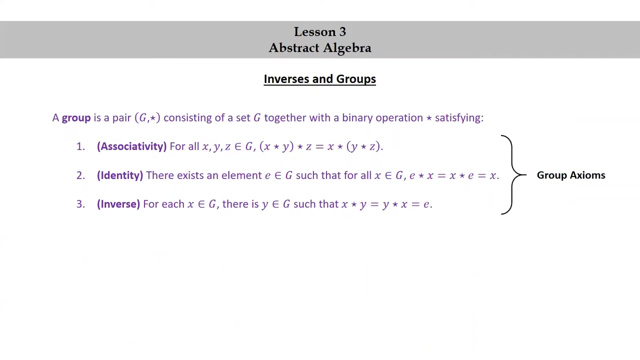 Two, identity. There exists an element E in G such that for all X in G E star X equals X star E equals X. Three, inverse. For each X in G there is Y in G such that X star Y equals Y star X equals E. the statements of associativity identity and inverse together form what is known as the group 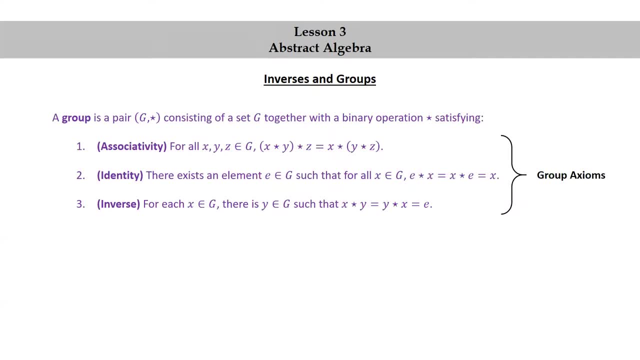 axioms axioms are just statements that we are taking to be true if y and g is an inverse of x and g we will usually write y equals x with an exponent of negative one that's pronounced y equals x inverse so x star x inverse equals x inverse star x equals e 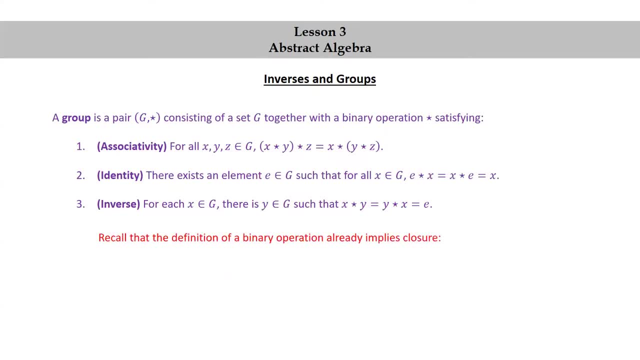 recall that the definition of a binary operation already implies closure closure says for all x y and g x star y is in g some authors will mention closure explicitly instead of using the expression